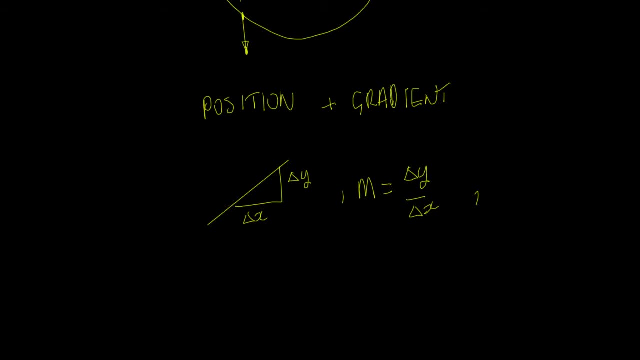 Or, if we want to, we could go to that point in the line and we could say m, and if we multiply m by delta x, Delta x, We will get delta y. we've just changed this equation. transpose this equation for delta y. now, if we had, 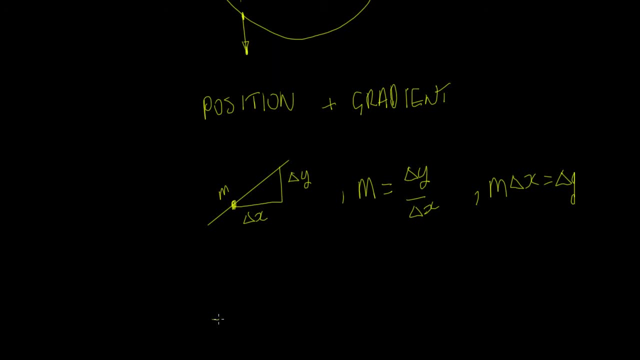 instead of a straight line, we had a curve. so there's a curve, now that's some function x, some function f, and that's x and that's y. then again, if we took this point here, the gradient at that point there would be given by df, by: 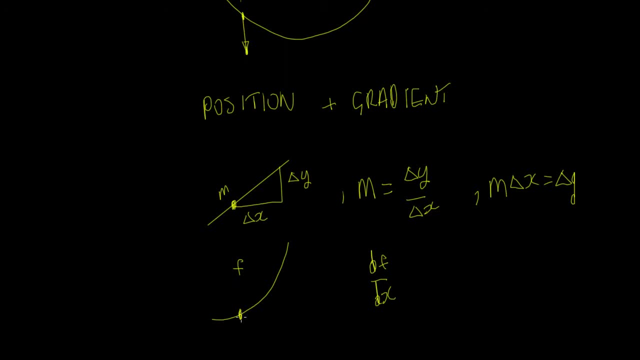 dx. so that's just the gradient, that point there. now, if i could draw it, i'll try, and i'll try and get the pen on there. let's just see if i get a line there. oh, let's get that up there. oh, there we go. oh, no, it's not. 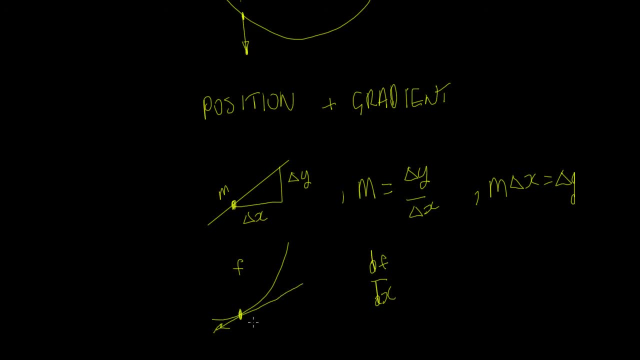 anyway, that's the gradient there. now if we take that gradient, that point there, and multiply it again by delta x- same delta x is there- then we'll get that little distance there. delta y. so we're taking that df by dx, multiply it by delta x, then we will get. 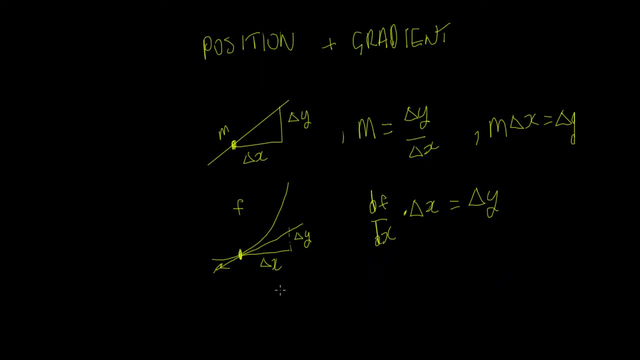 delta y. now also, if you were to swap the axis here, and if you made that axis there the x axis and you made that axis there the y axis, then you could write that equation as df: by dy times delta y would equal delta x. all we've done is changed the. 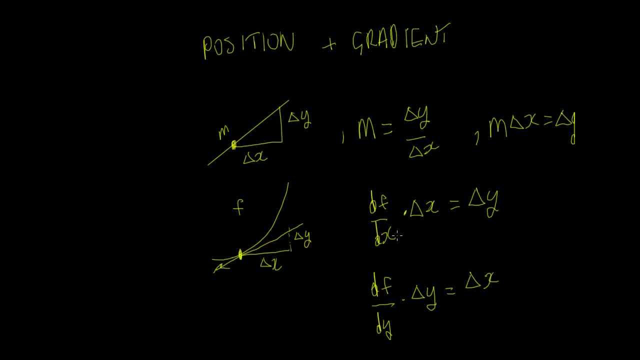 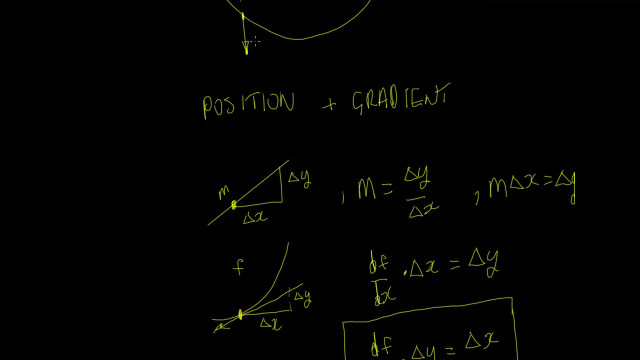 the way the graph. the graph is written. it's just a and all the real realness. all we've done is just changed the the letters here. so if we remember that, okay, now, when we change this position here, what we're doing is we're changing the function. 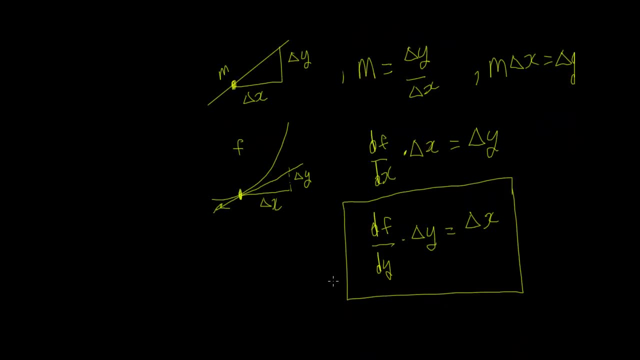 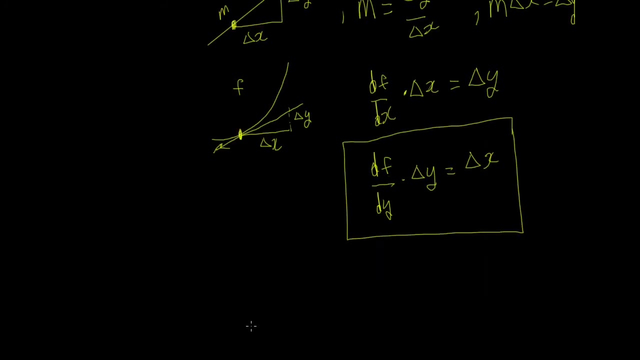 df by dy and if we multiply that by a small change delta y, we will get our delta s. so let me just write that out again so you understand. well, actually we're doing it in terms of this example. so right, in terms of the potential, energy equation, energy potential. 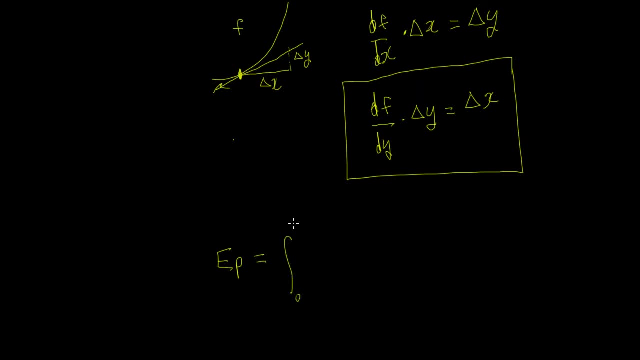 equals that integral from zero to l of y of x times root of one plus y, derivative of x squared dx. right now we don't really need these at this integral sign, because what we're doing is we're looking at a localized phenomenon, we're looking at the 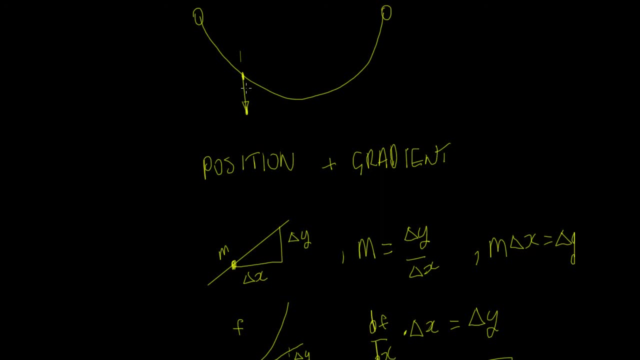 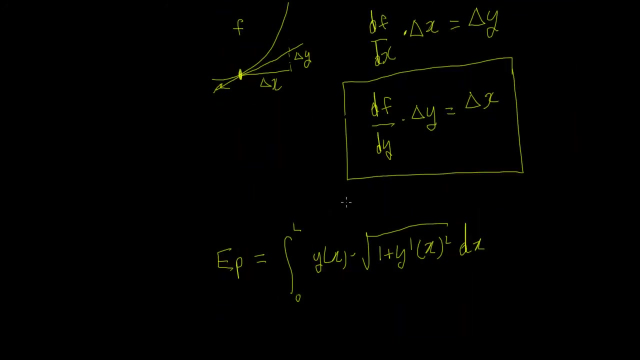 the change here when we keep x constant. so we're not adding up any of this, we're just looking at one infinitesimal point, so we don't really need to look at it in terms of that integral. so this here: if we call that our function f, then what we would have we would have when we move that. 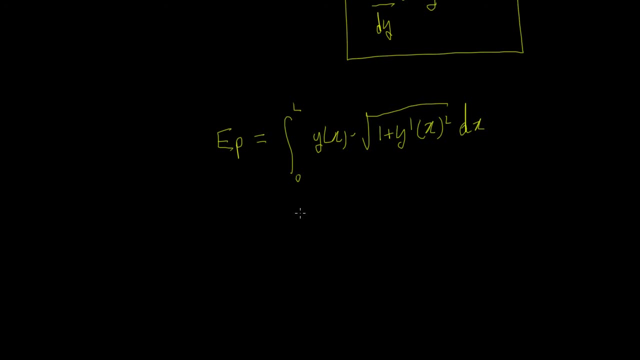 rope down the way, we would have a partial f by partial y. that's partial f by partial y because we've kept x constant, and if we multiply that by delta y, then what we'll get is the change here in terms of the energy potential. so we're going to have delta.